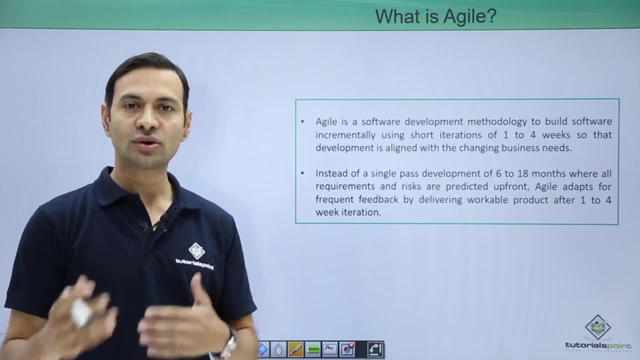 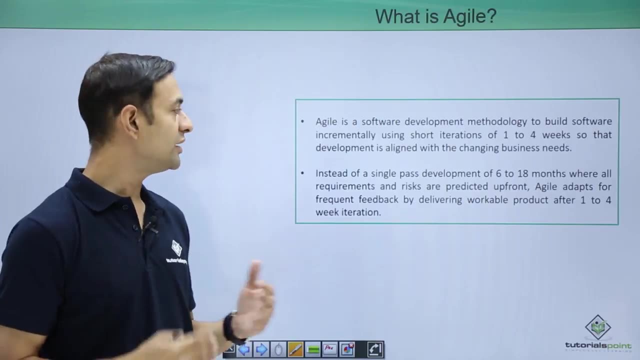 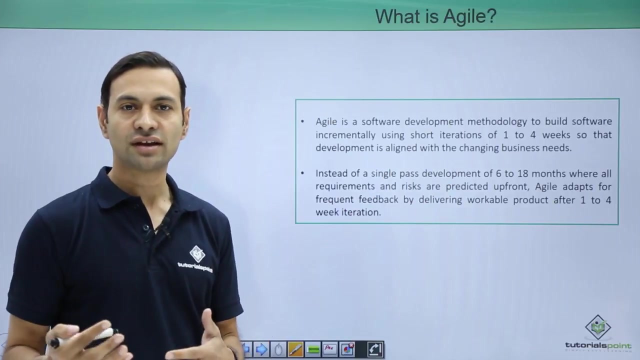 you need to incorporate those changes in your software development during software development life cycle. So Agile basically works in that way. Agile is a software development methodology to build software incrementally using short iteration of 1 to 4 weeks so that your development is aligned with the changing business needs. Changing business needs says within a software. 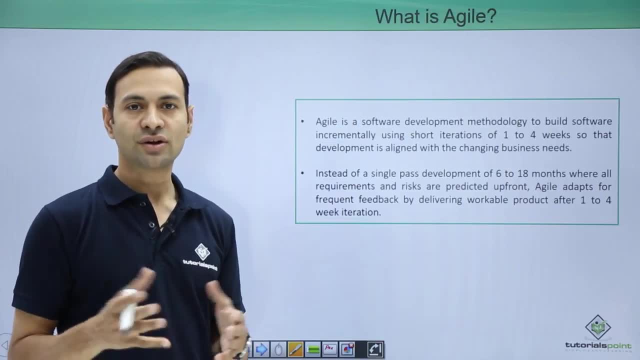 development. you are like in made of software development and client says: no, sir, I want these changes to be done within software, in this software, Otherwise my software will be rendered useless. But you are in made of software development. you know okay at this. 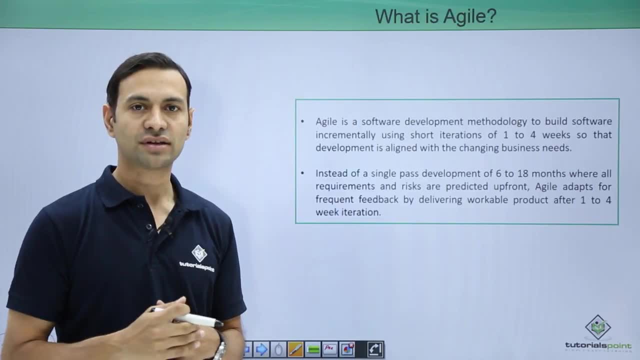 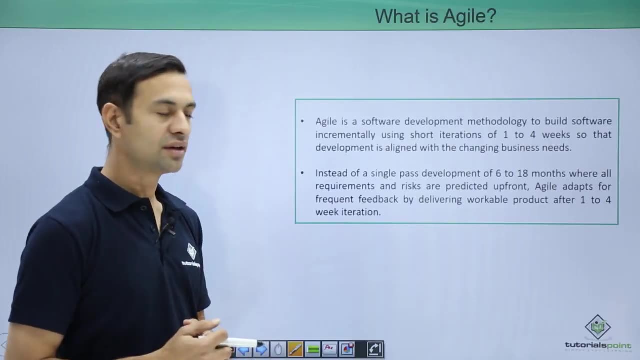 point of time, if you change something, that is a huge impact. So how to deal with it? Agile deals with such things. So instead of single path development of 6 to 18 months where requirements and risk are predicted upfront, Agile adapts for frequent. 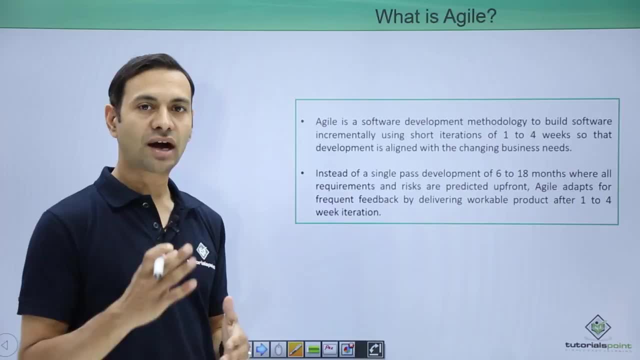 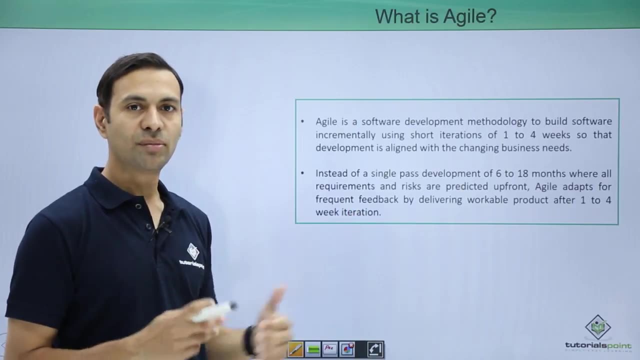 feedbacks by incorporating changes after every 1 month or half a month. So we have workable product after every 1 to 4 weeks of iteration. Basically what we do: we make a check to the client. Okay, sir. 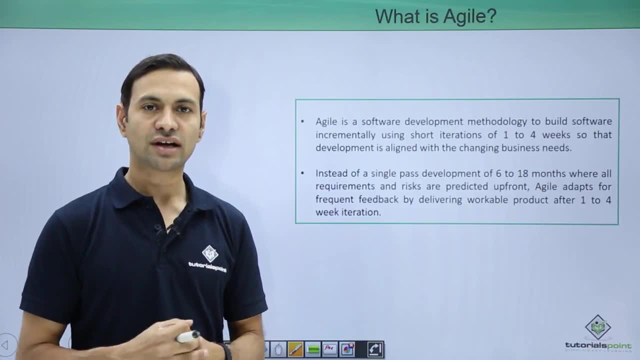 So far we have developed this product. Can you give feedback on it after a month of development? Client see: okay, things are going in line with my requirement, then you can go ahead. Oh no, I need the changes. make the changes in the product right now so that later on. 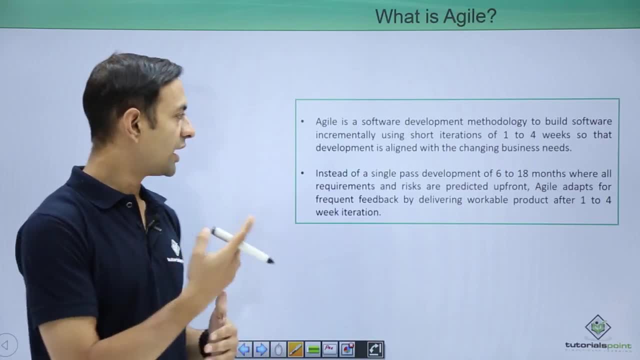 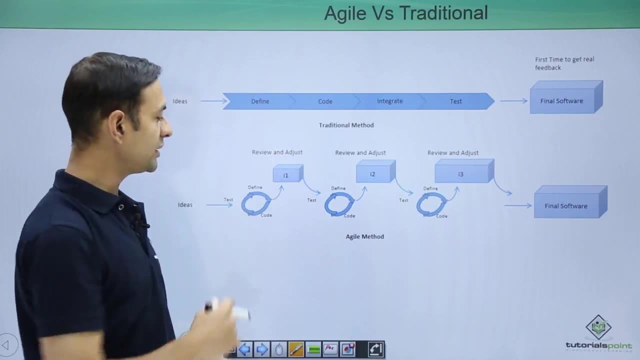 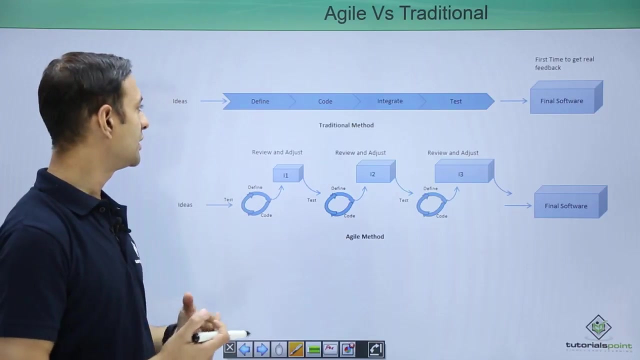 I may not feel disgusted. So let us see how my Agile works structurally. So here we are basically with the traditional method of development and Agile method of development. In traditional method we have ideas, basically requirements. we have received from clients basic requirements. 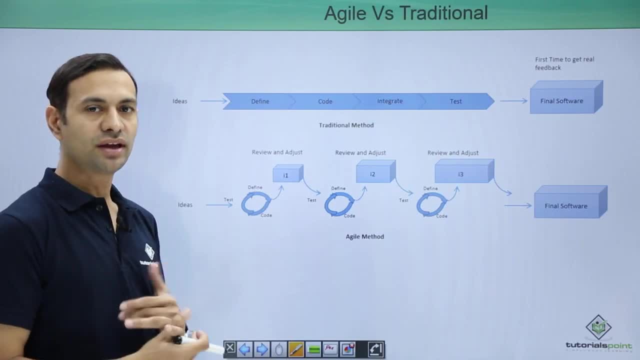 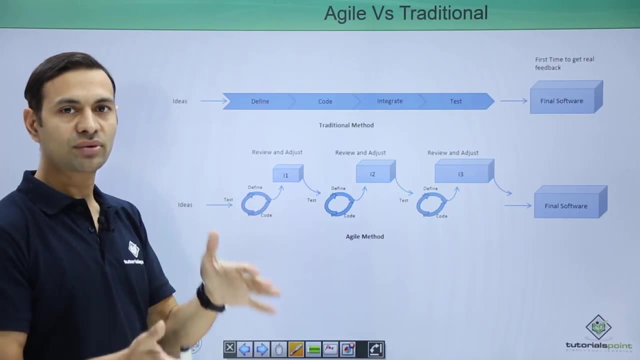 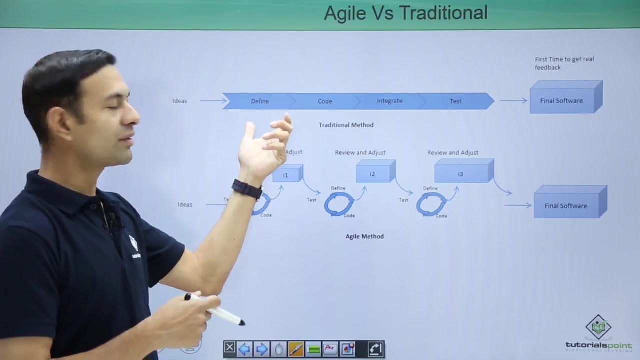 because clients say, okay, this is I want to do. how to do is our responsibility how to make it done? So we have ideas from clients. we define it. okay, the set of requirements make documents with hundreds of requirements written in a short and crisp way. then we define our code. 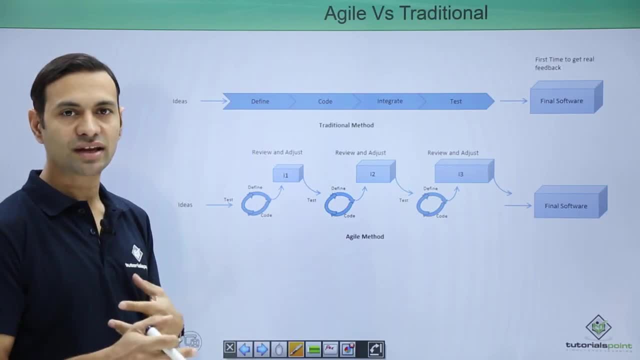 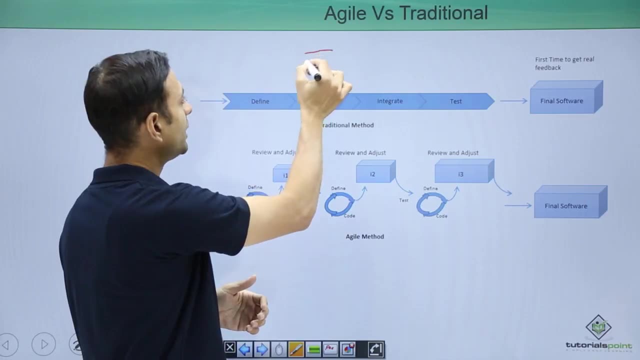 we plan it, okay, what to do, how to do. we do class diagrams, everything. then we code it, then we integrate: Okay, And coding is done by multiple teams. Say there are five teams, we, they are doing code. 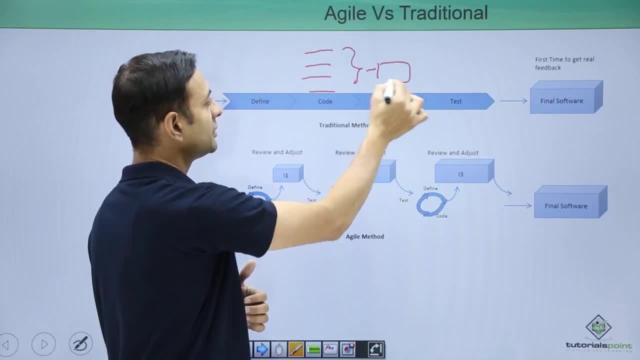 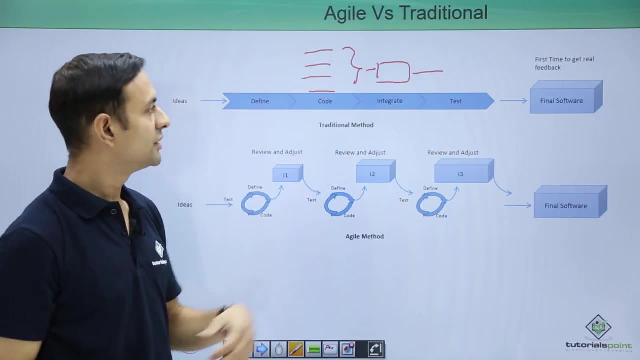 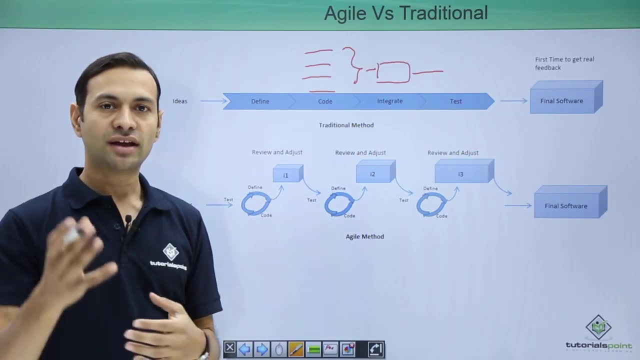 then we integrate their code, then our product gets ready, then testing team test it and then final software gets prepared. So it is the first time to get the real feedback from the client. After one and a half year of time we have developed the complete product. 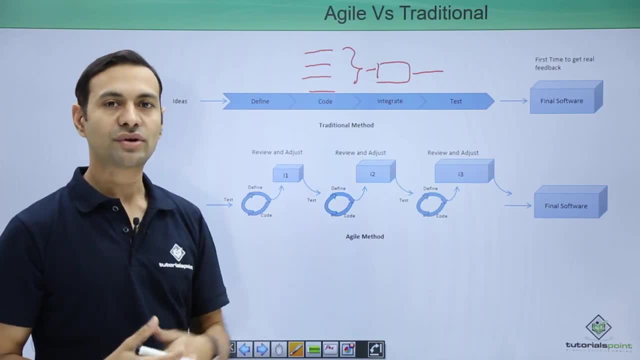 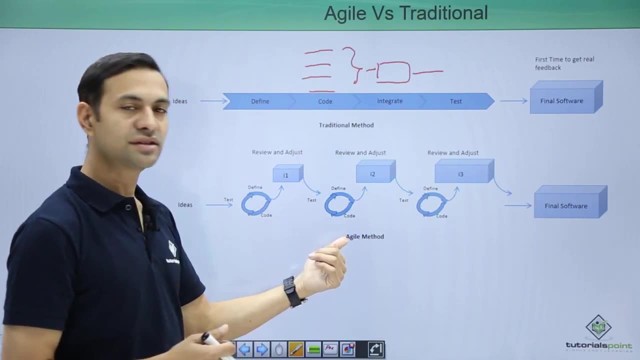 give it to the client. okay, sir, please check if it is meeting your requirements or not. So there is no option of feedback. So we have no option of feedback in between this particular software development cycle. So agile works in that way, okay, No, sir, you are not required to give feedback after. 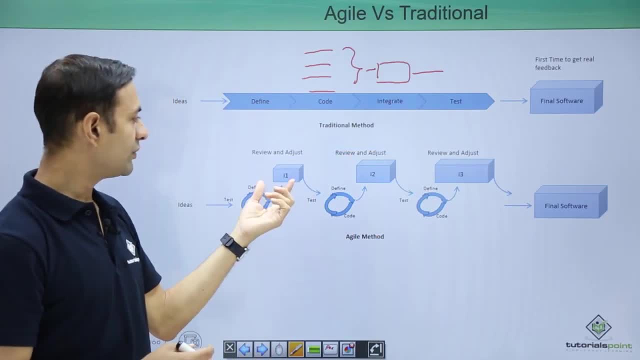 the product is developed, You can give me feedback. I will give you incremental development. So I am developing few set of requirements instead of all requirements at one time. So how things are done: you get the ideas from the client, then we have a cycle, we fix. 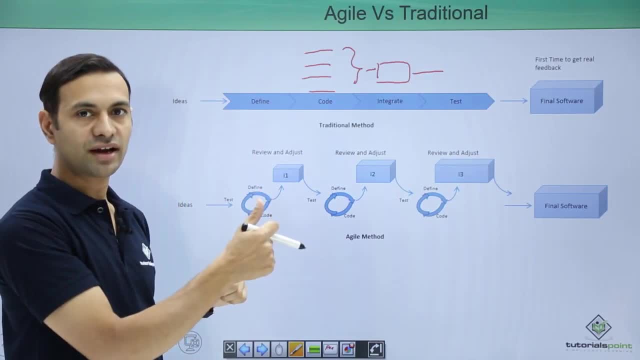 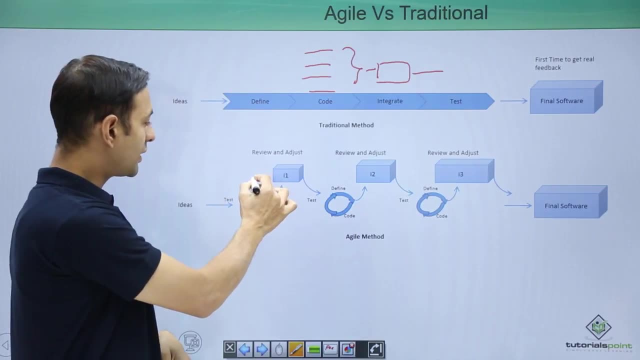 okay, We are, instead of making all set of requirements done one at a time, we are taking few set of requirements, we code them. we define the requirements. okay, these requirements are to be done. we code, then test it. A small set of product is developed, it is given to. 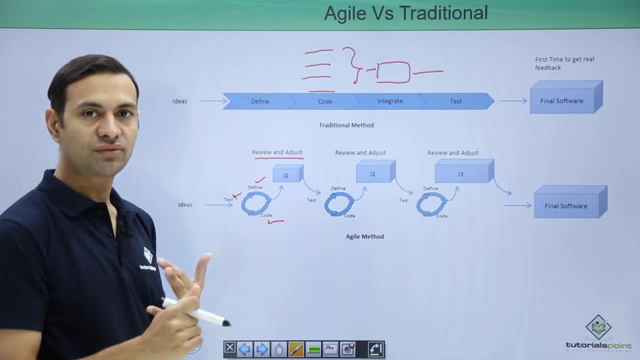 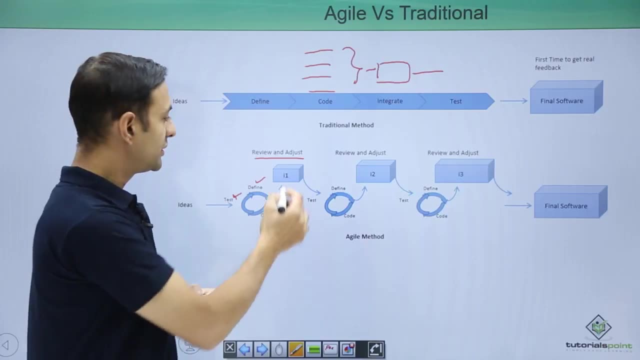 the client to test it. who test? who take the feedback? we take the feedback. okay, client is given certain feedback. so we change the products, review and adjust. okay, So we make adjustments. then another set of requirements are made. we have set of requirements which. 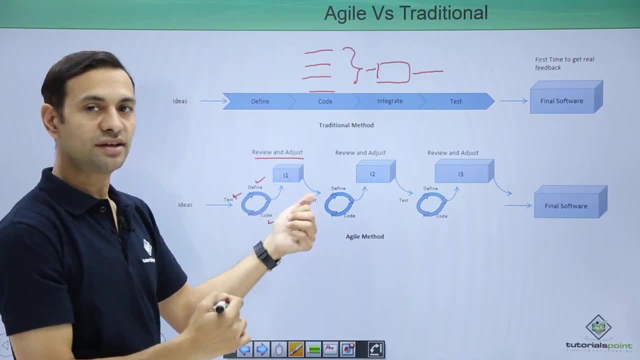 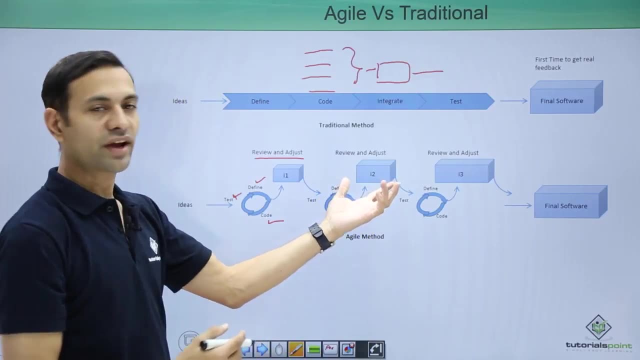 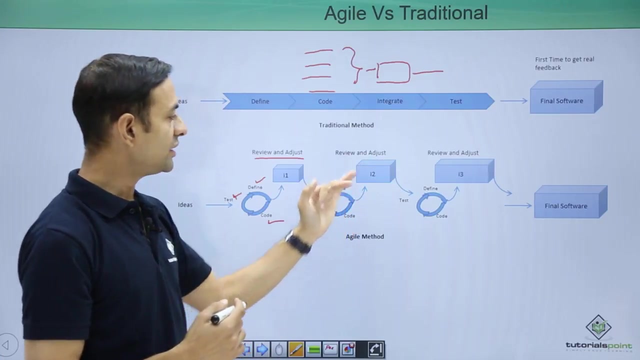 are new and set of requirements which are to be adjusted. then this cycle refines further and your product is second iteration. It is further refined, You see the bigger one. Now again it is sent to client review. we make adjustments, then another iteration again. 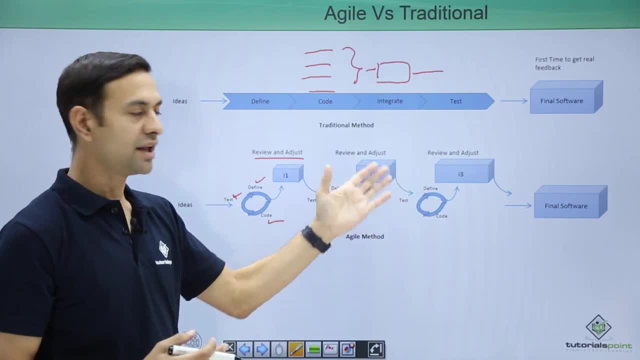 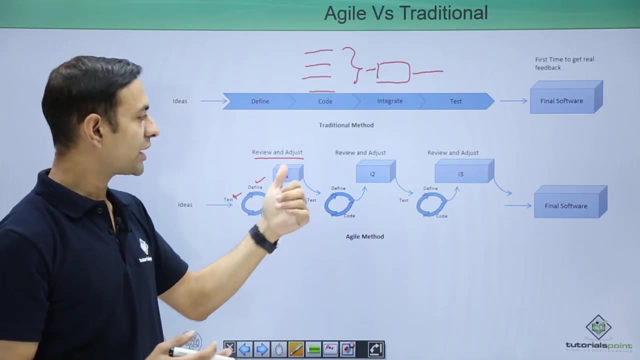 so we are refining our product, we are enhancing it day by day, we are reviewing it, adjusting it and finally the software once received, to the client. he has already given multiple times the feedbacks, So we have incorporated client changes in each and every month. So that's way how agile works.